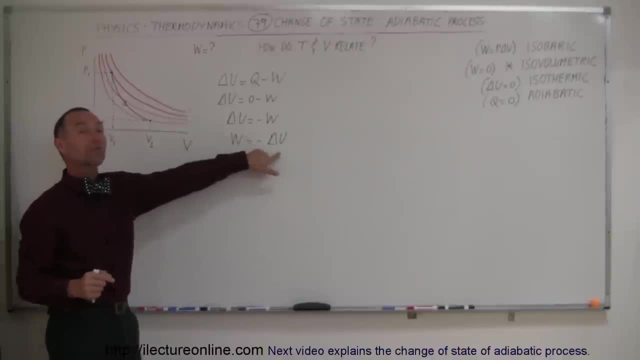 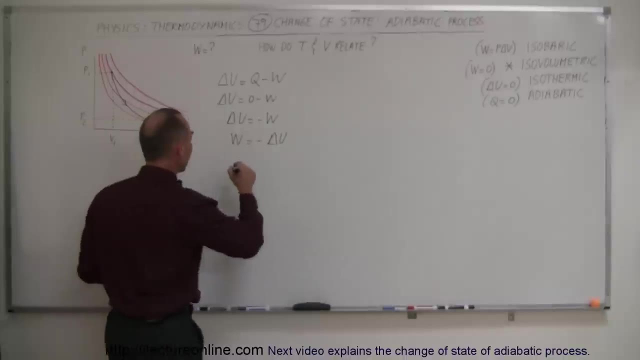 that's exactly what it says. however much work you do, you're going to take all of that work, all the energy to do the work out of the internal energy of the gas. and remember the equation for the internal energy of the gas is that W is equal to minus, of course the minus is still there, and C 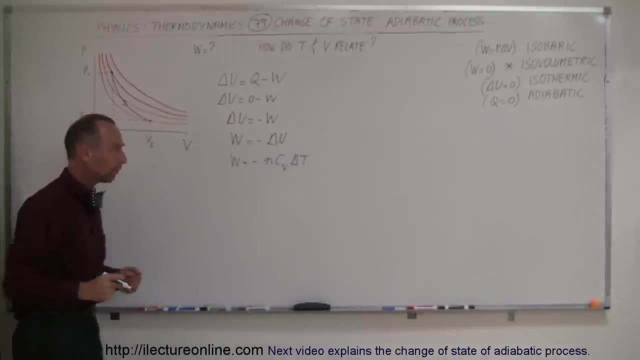 sub V times, the change in the temperature, delta T, and so for us to figure out what the work is, what the work is that's done by the gas, we have to go ahead and figure out what the change in the temperature is, know what the C is for the gas, the constant volume, specific heat and, of course, the 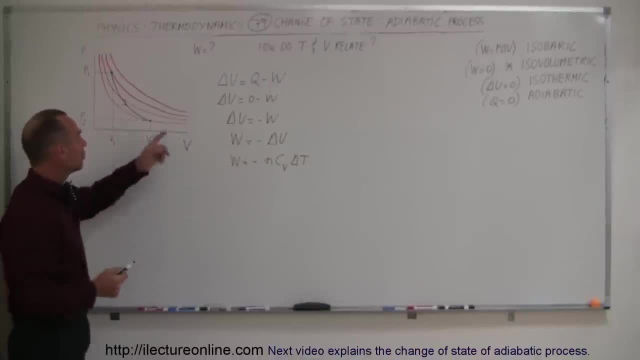 number of moles. The problem with an adiabatic process is that you're not going to know what the temperature change is. that's going to be difficult. we have to find a way to somehow relate the temperature to the volume. you can see as the volume changes, the temperature changes as well. and 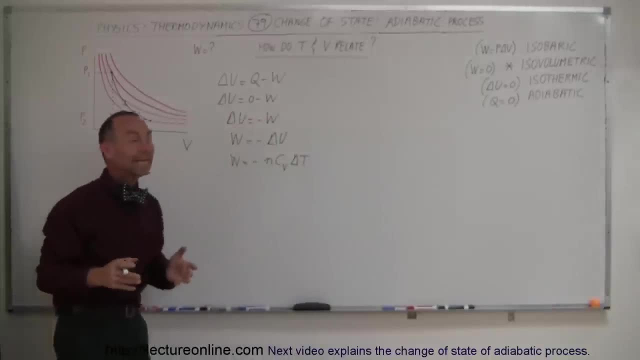 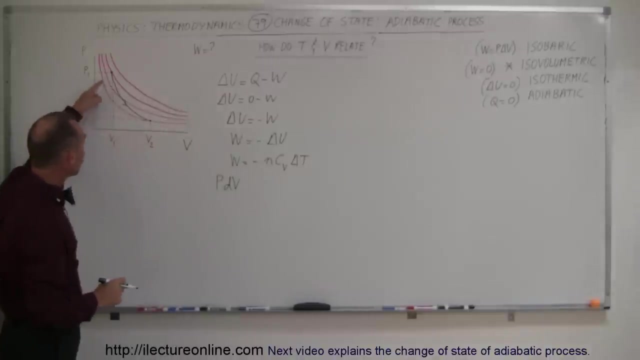 so the question then comes up: how do the temperature and the volume relate in an adiabatic process? Well, the way we do that is the following way. So, first of all, work typically is equal to the pressure times, the change in the volume, and I'll just write it as dV because, again, since the pressure changes through the process, we 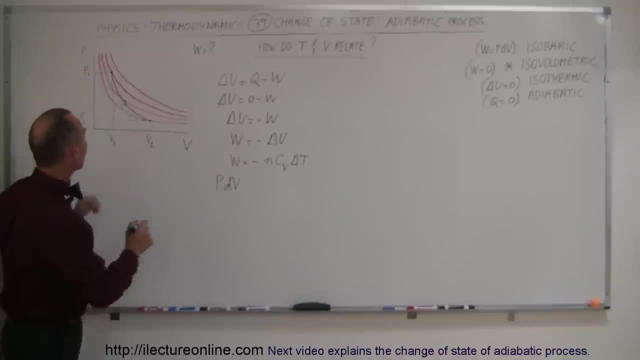 have to take a small, infinitesimal step. and so we're just going to go to a very small step within the process of this, this process change, and so write as p times delta V. and then here we're going to write this as minus n, C, sub V times dt, because, again, over a very small portion of the process change, we only change. 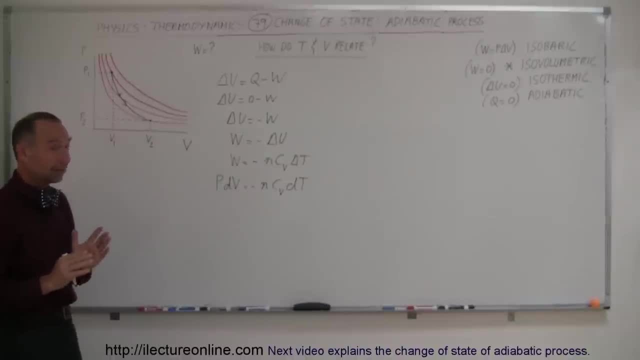 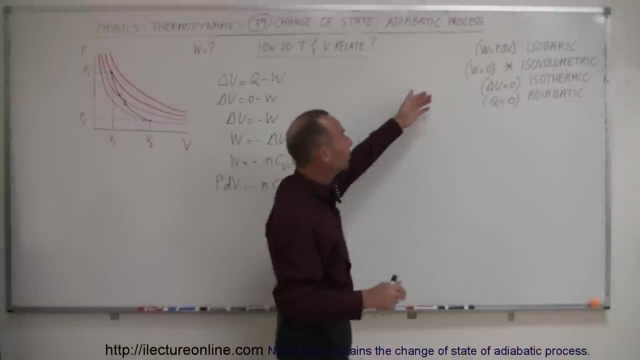 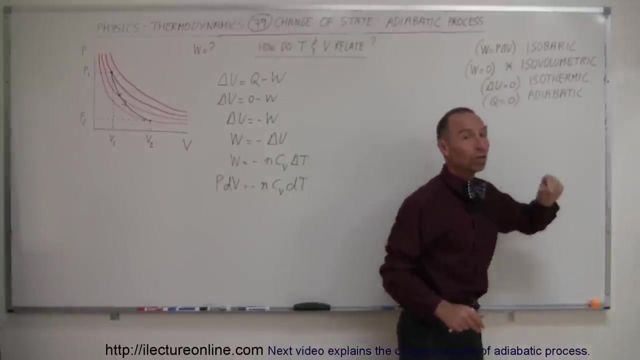 the temperature by a very minute amount. Now we realize that in an adiabatic process pressure, volume and temperature all change. in the three other processes one of them stayed the same: here pressure didn't change, here the volume didn't change and here the temperature didn't change. so only two of 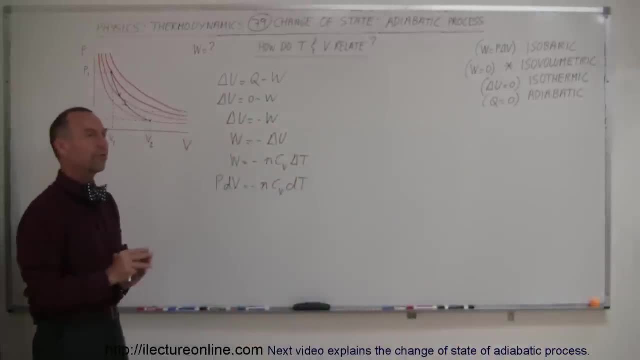 the three variables changed. but in an adiabatic process all three variables change, Wow. so, and how did they change? because you know if one change is going to affect the other two. so there's got to be some sort of relationship between temperature, volume, pressure, volume and so forth, and we're going to figure out how to do that. So the next thing we're 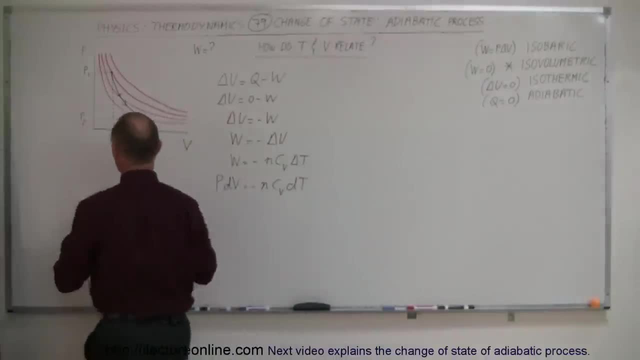 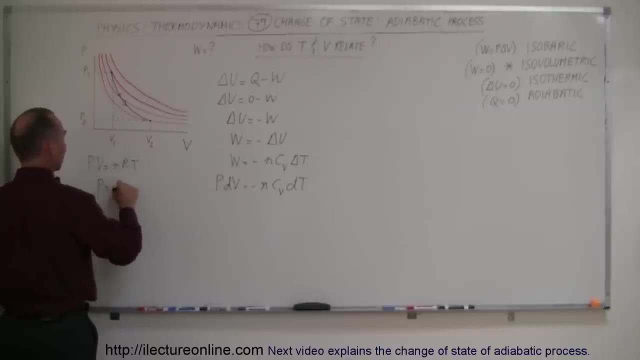 going to do is come up with the gas equation. let me write that over here. so we have pressure times. volume is equal to nRT, which means that the pressure is equal to nRT divided by the volume, and we can go ahead and plug that in. 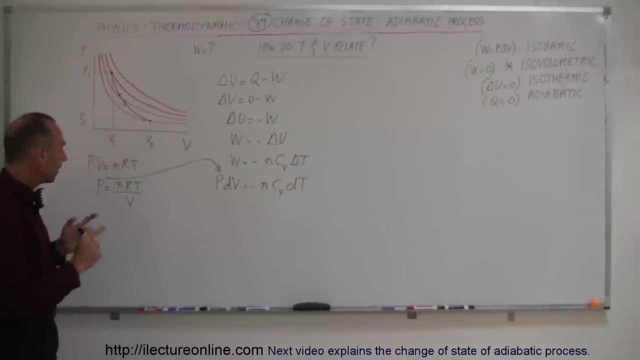 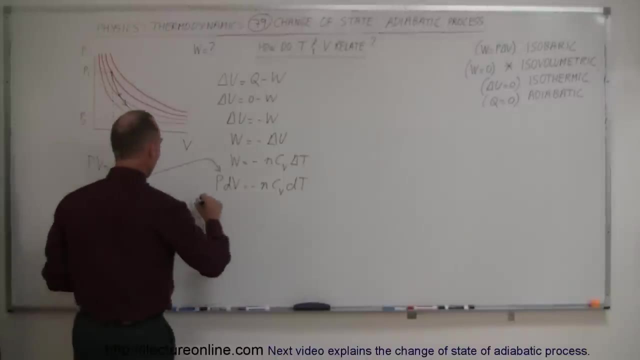 into our equation right there. So by doing that I've eliminated one of the three variables and now have an equation with only two variables, which is easier to solve. So let's plug that in. so now we have: nRT over V times. dV is equal to minus nC sub V times dt. All right now notice that I have an n on this side, an. 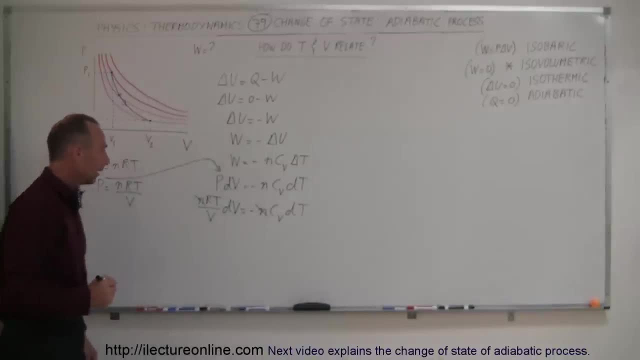 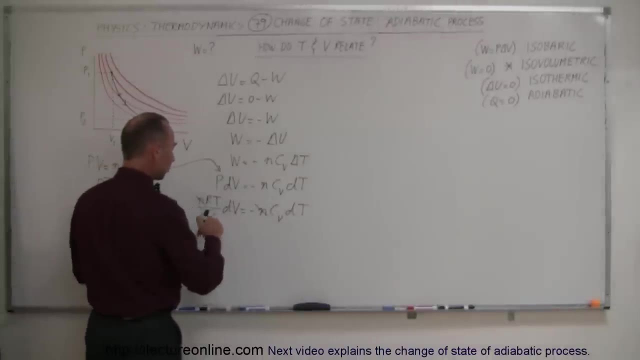 n on that side, and they can definitely cancel out What else? well, so far that's it. Now, what I'm going to do is I'm going to put the t down here and the v down here, so now it looks like r times. 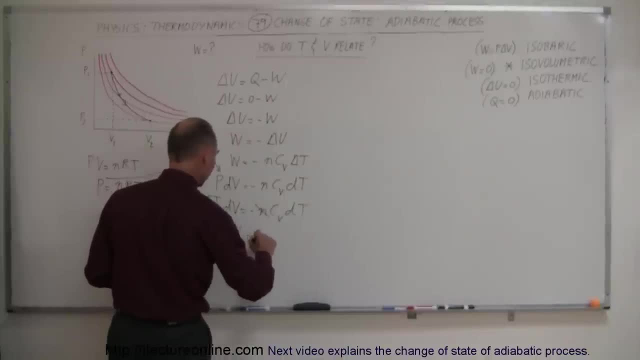 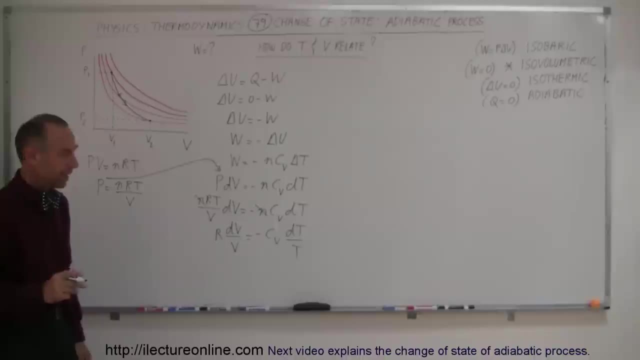 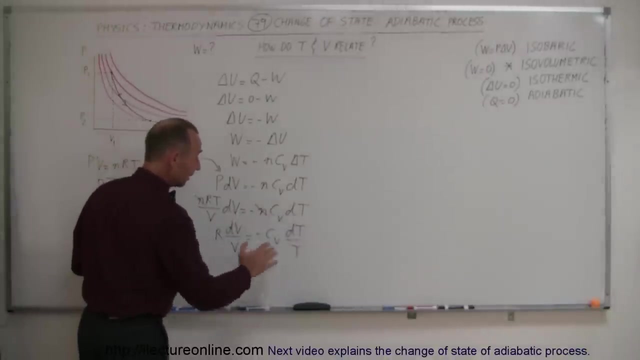 dv. dv over v, there we go- is equal to minus c sub v times dt over t. Ah, now we look like we have a differential equation and we can go ahead and integrate that, because we have a dv and a v here, a dd and a d there. so we know we can integrate that. but before 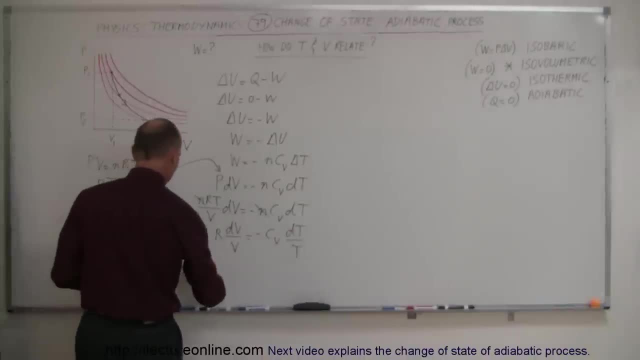 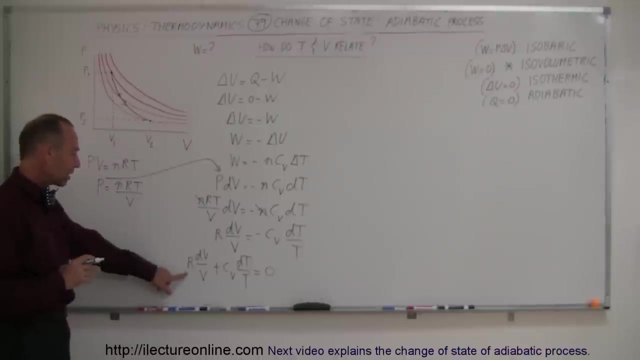 we do that. to make it simpler, I'm going to move everything over to one side. so now we have r times dv over v plus c sub v times. dt over t is equal to zero. Before I integrate, I'm going to do one more thing. I have an r here and have a c sub v here and there. 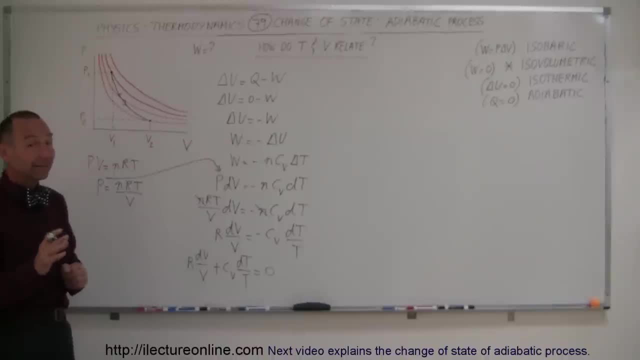 is a relationship between c sub v and r and c sub p. Let me illustrate that here. We know that r really is the difference between c sub p and c sub v. If I subtract c sub v from c sub p, the difference for any gas, be it monatomic, diatomic, triatomic, the. 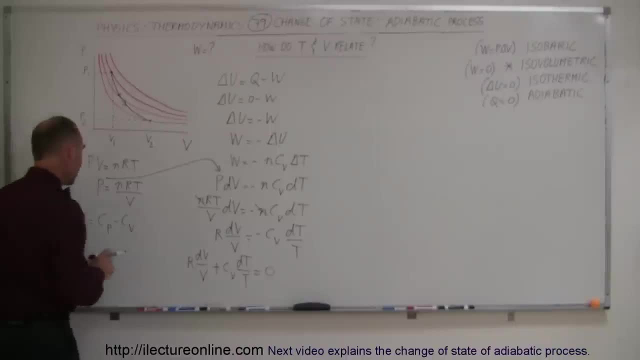 difference between the gas is always equal to r, so which means I can actually replace r by c sub p minus c sub v. Okay, I can go ahead and do that here, or maybe I'll leave it until later. I'll just keep that for now and leave it until later What I'm going to. 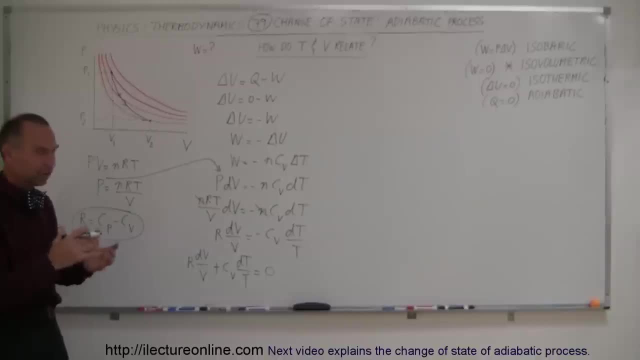 do now is I'm going to integrate both sides of the equation. Of course, the integral is zero, still zero, or if this is equal to zero, then I can integrate and still get it equal to zero. We're good there, Let me do that. then I'm going to integrate the left side, like so: 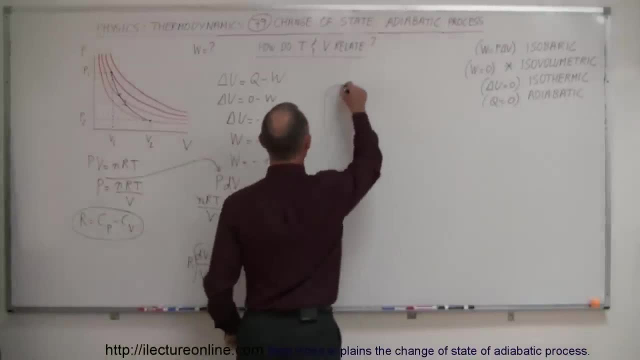 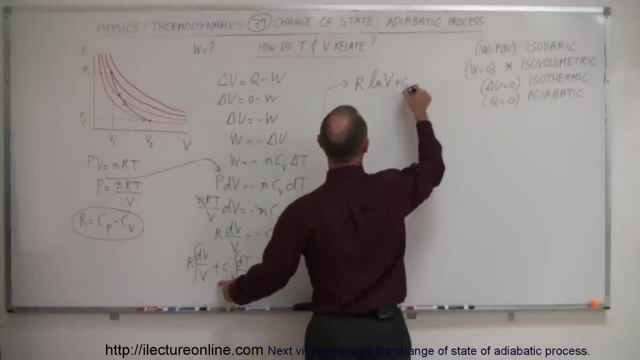 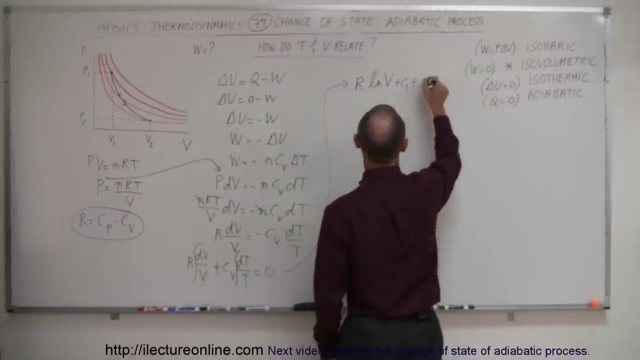 and what do I get when I do that? All right, let's come over here and we have r times, the natural log of v. Of course we have a constant of integration. We can't forget about that. Plus- and I'm kind of running out of room here- c sub v times, the natural log of. 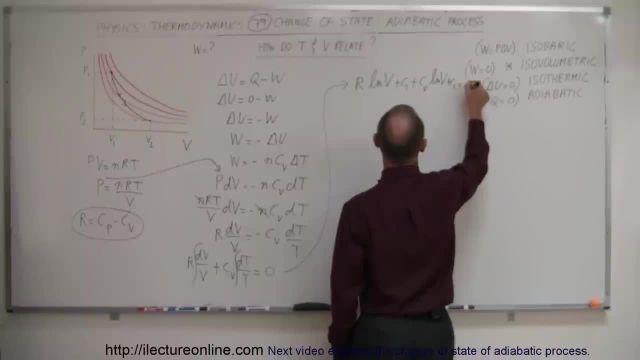 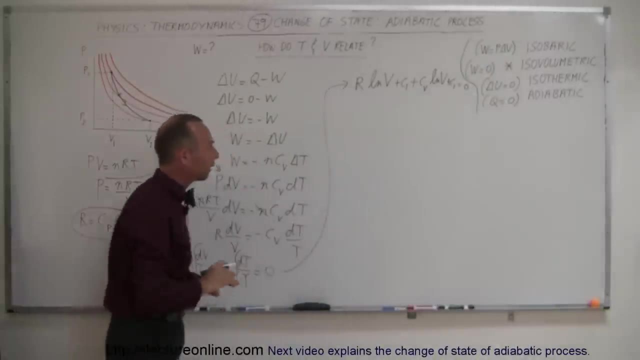 v plus a constant of integration, and that, of course, equals r. So we're going to do that. So our full d of r, times d of d greater than or equal to the r times d of d greater than, of course, equals zero. Now, actually, technically speaking, 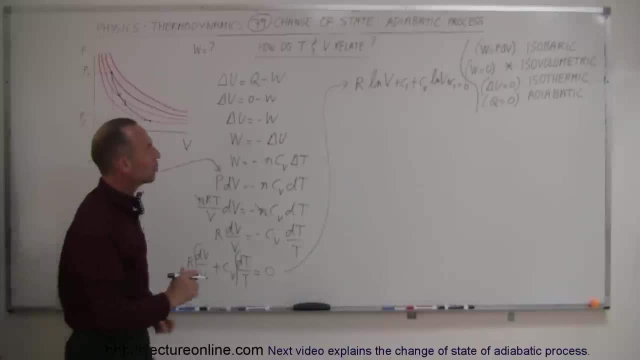 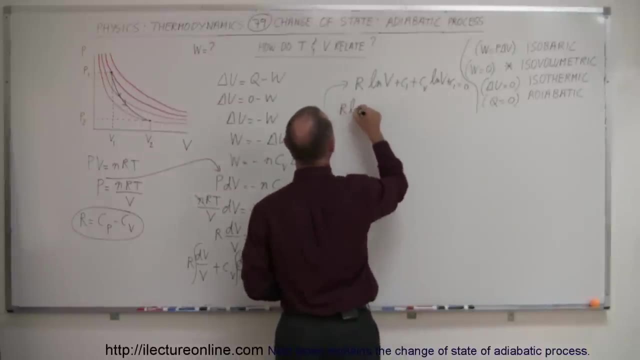 to integrate zero. we probably should get something as well, But that is taken care of by the constant of integration on the left side, so we don't have to worry about that. All right, next thing we're going to do is move the constant of the integration to the. 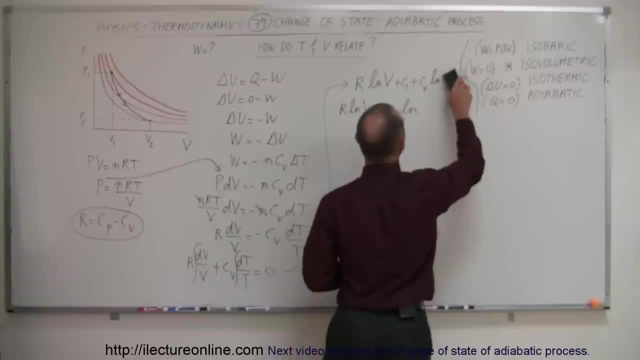 other side and combine them. So now we can say that r times the natural log of v plus c sub v times the natural log of. oh, this should be t. I've got the wrong variable over here. It should be temperature, So this is temperature. So natural log of temperature is equal to a constant. 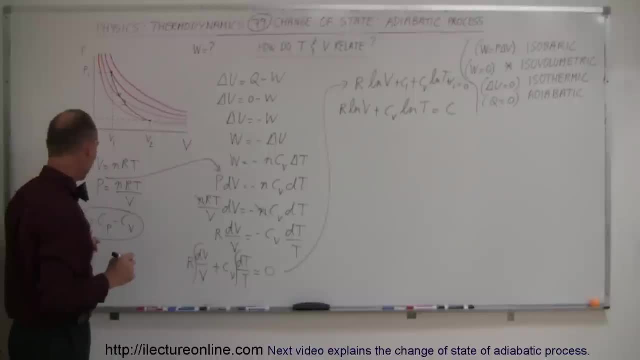 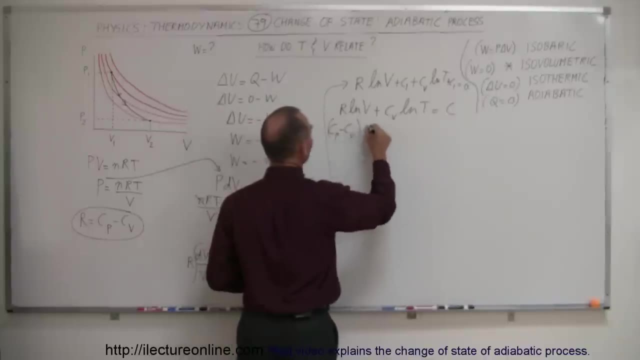 Okay, now I'm going to go ahead and plug this thing in right here. So I'm going to replace R by C sub P minus C sub V. So we have C sub P minus C sub V times. the natural log of V plus C sub V times. the natural log of T is equal to a constant. 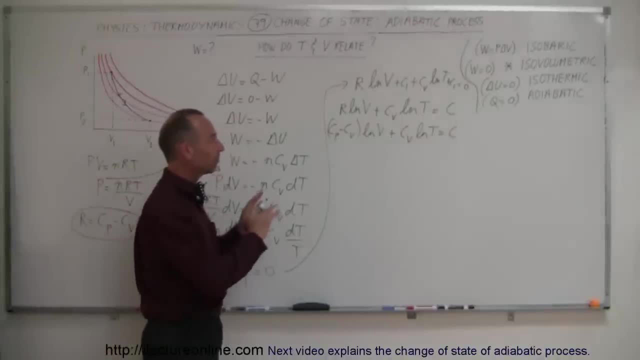 Now the next step is kind of a mathematical trick. We have to somehow get this equation to look in such a way that we can relate T and V to one another. So how do we do that? Well, the trick is to divide all three terms by C sub V. 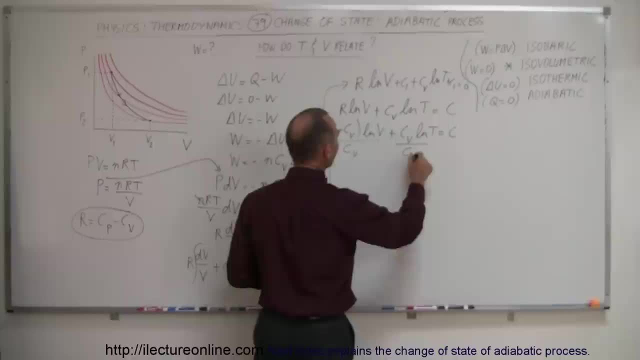 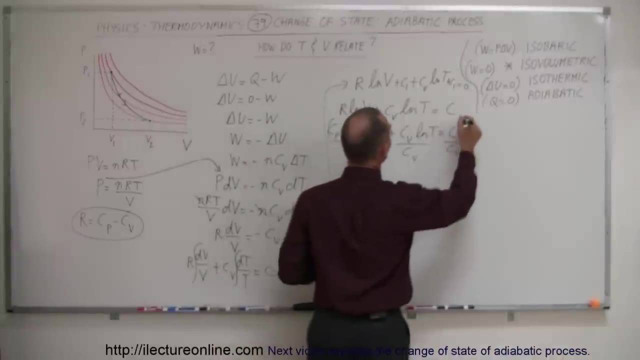 Now C sub V is simply a constant. so we divide this by C sub V, divide this by C sub V and divide this by C sub V And, of course, a constant divided by another constant is still a constant. So just to keep things separate, I can call this constant 3,, constant 3, and if I divide this into that, I still get a constant. 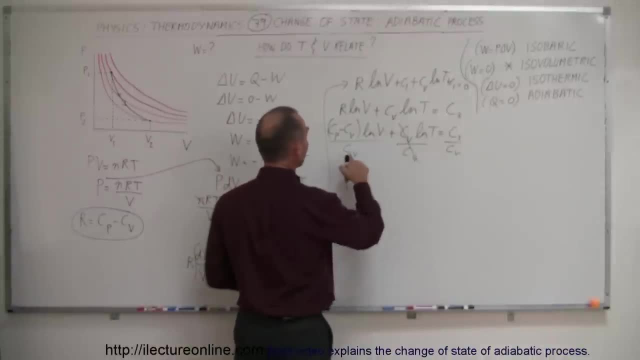 All right, but that will cancel these out. And then, if I divide this into here, what do I get is I get the following: I get C sub P divided by C sub V, minus C sub V divided by C sub V, which is 1,. 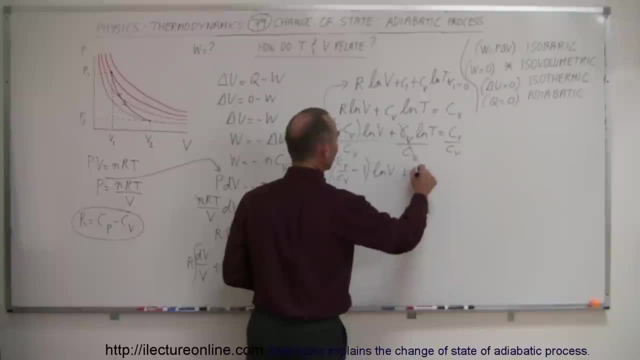 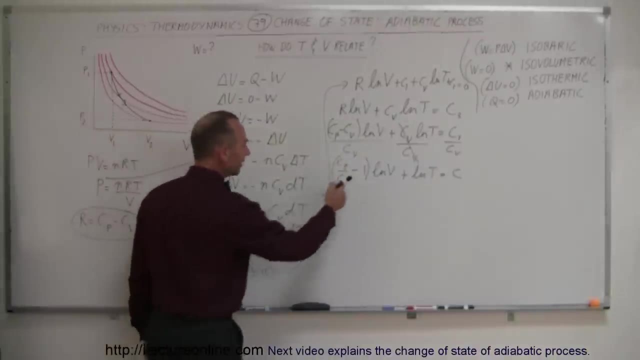 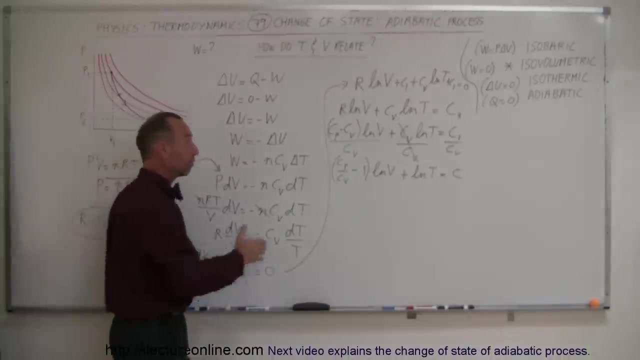 and multiply this times the natural log of V plus the natural log of T, is equal to just another constant. Now what we're going to do is we see this ratio here: C sub P divided by C sub V, and that ratio is different for different gases, because for monatomic gas, 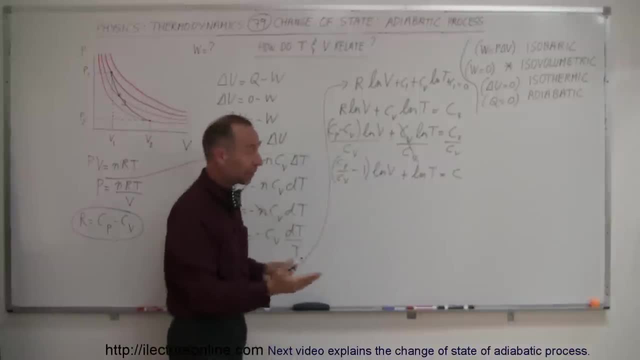 this is 5 halves R and this is 3 halves R, and for a diatomic gas this is 7 halves R and 5 halves R, and so forth. So even though that ratio is different for different gases, we still take C sub P divided by C sub V. 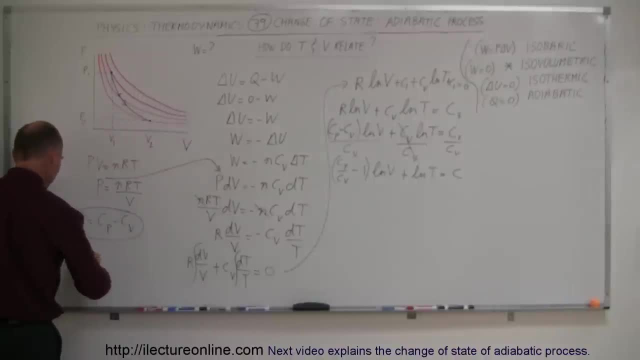 and give it another variable, give it another variable name. We call that gamma. Gamma is now going to be defined as C sub P, divided by C sub V, and we're going to replace that into our equation over here. So now our equation looks like: gamma minus 1 times the natural log of T. 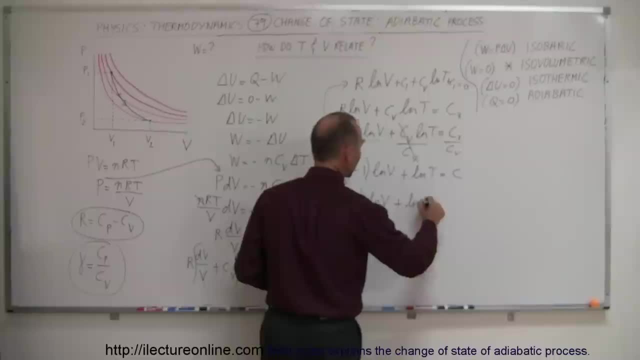 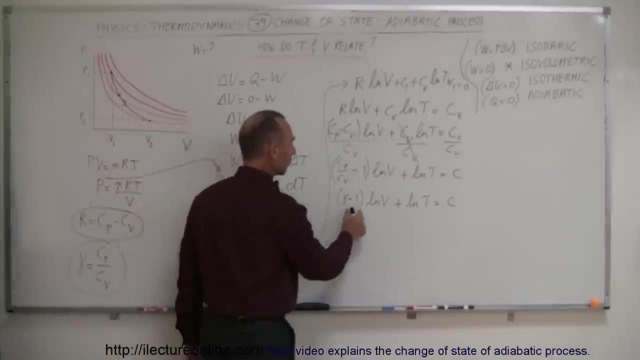 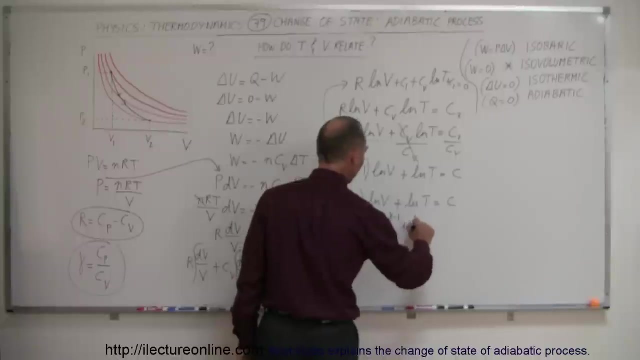 times the natural log of V plus the natural log of T is equal to a constant. Now we're going to use the laws of logarithms. If we multiply something times a logarithm, we can make that the exponent. So this now becomes the natural log of V to the gamma minus 1 plus the natural log of T. 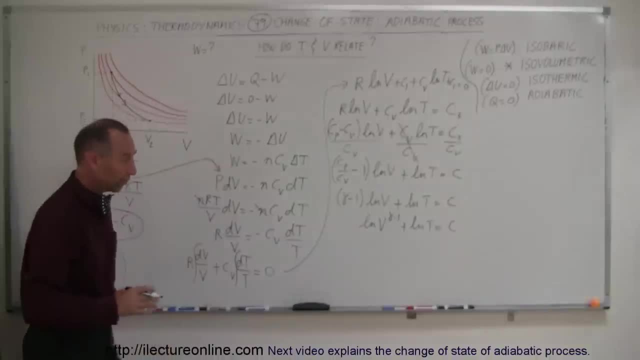 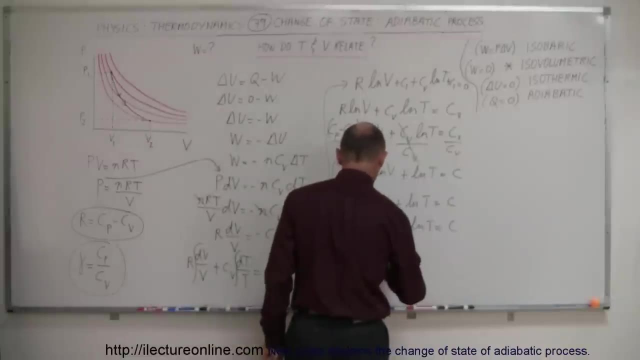 and we can set that equal to our constant. still, And now. the next rule for logarithms is that if we add logarithms together, we can actually write this as a product of the two terms in there. so we can say: this is equal to the natural log of T times V, to the gamma minus 1 equals C. 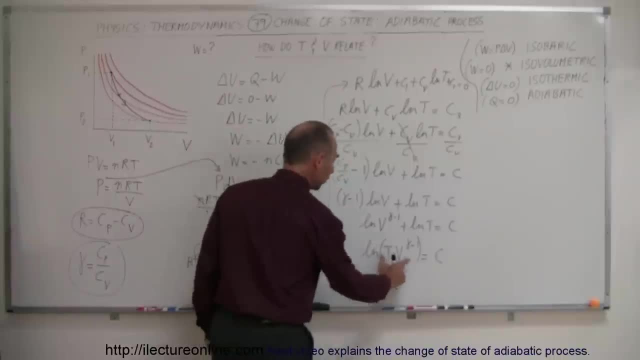 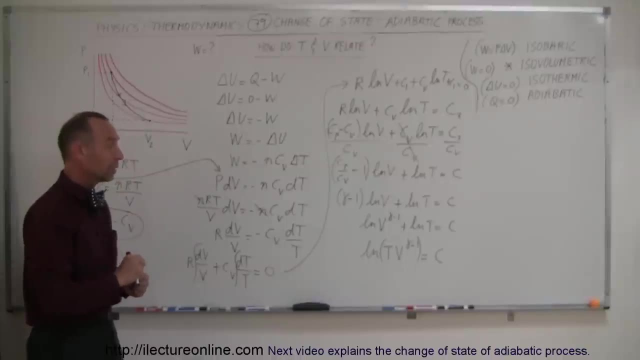 And let me put parentheses around this. So now we're taking the natural log of this whole thing. We simply put them together and multiply them together. So now, if the natural log of T times V to the gamma minus 1 equals a constant, 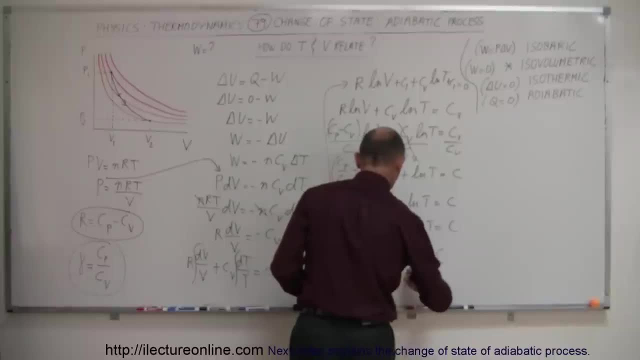 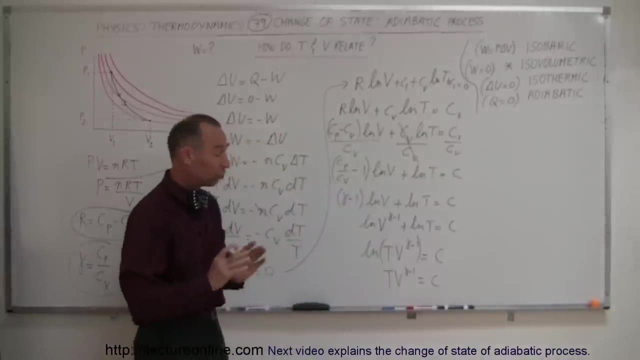 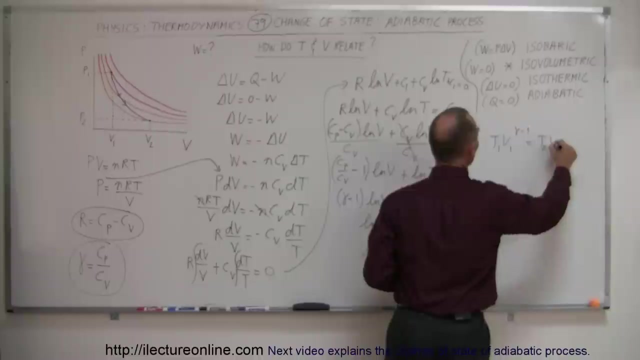 that means that T times V to the gamma minus 1 equals a constant. Of course, that's a different constant than that, but still represents a constant. And if that is true, then what we can say is that T1 V1 to the gamma minus 1 equals T2 V2 to the gamma minus 1.. 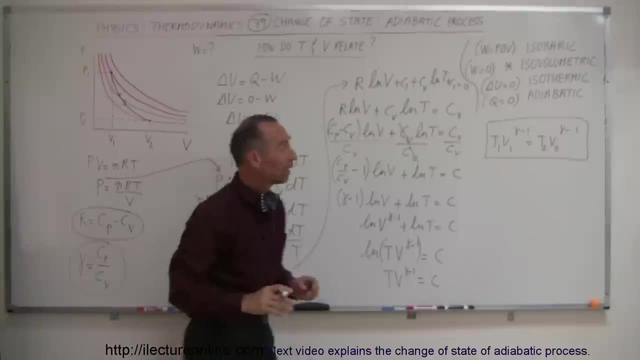 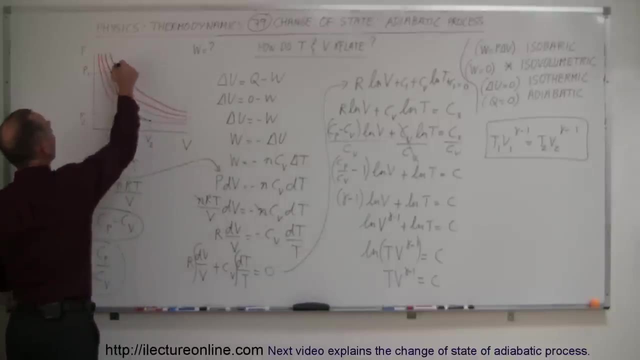 And here we finally have the relationship between temperature and volume in an adiabatic process. So if we take our beginning point and call that point number 1, and we take our end point in the process and call that point number 2,, 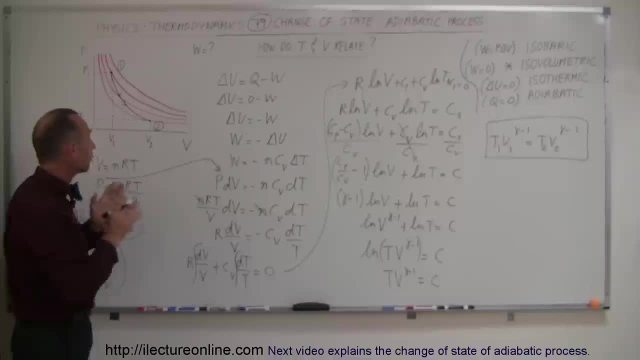 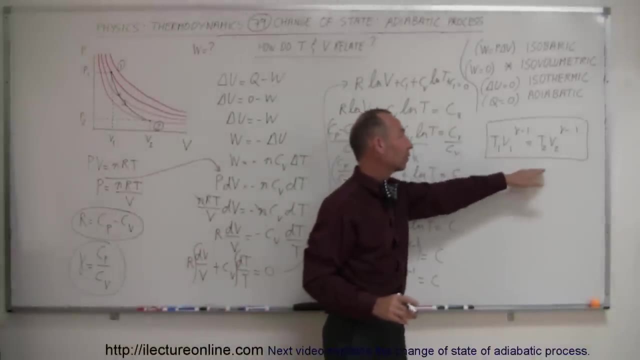 we can then say that going from 1 to 2, the temperature and the volume relates between those two points in the process. is this right here that T1 V1 to the gamma minus 1 equals T2 V2 to the gamma minus 1.. 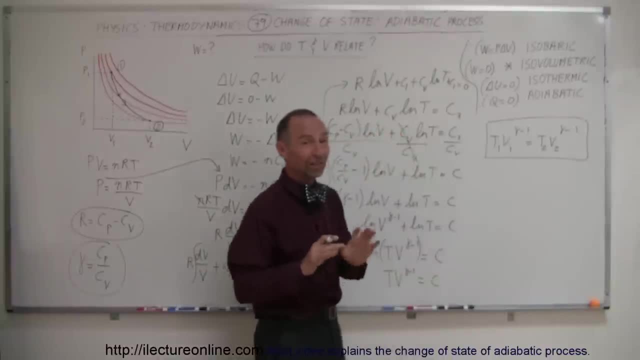 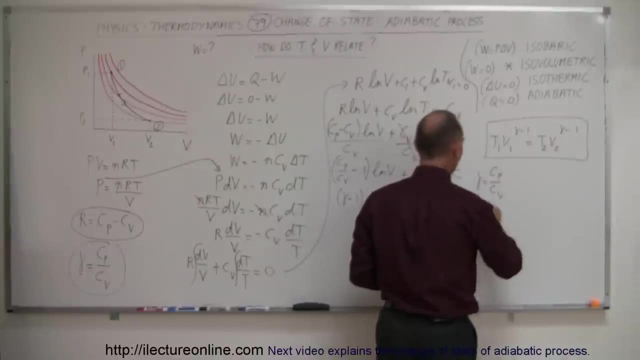 Now, that gamma symbol still probably confuses some of you, so let me explain that. So gamma is equal to the ratio of C sub P divided by C sub V. And for a monatomic gas, let me give myself just a little bit more room here. 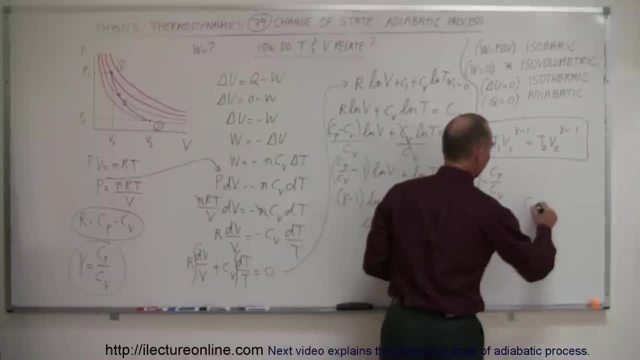 So for a monatomic gas- monatomic- let's see what C sub P and C sub V is. Let me go C sub V first, because that's a smaller number. So C sub V is C sub P. So C sub V is 3 over 2 R for a monatomic gas. 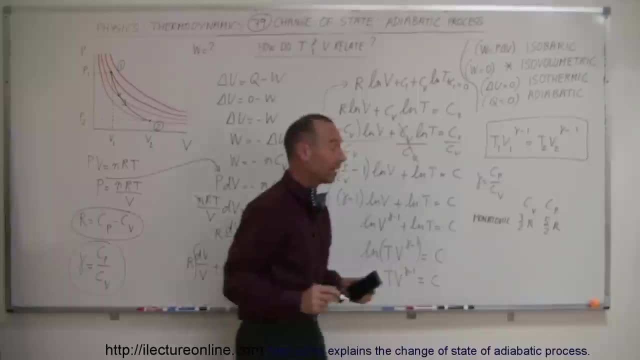 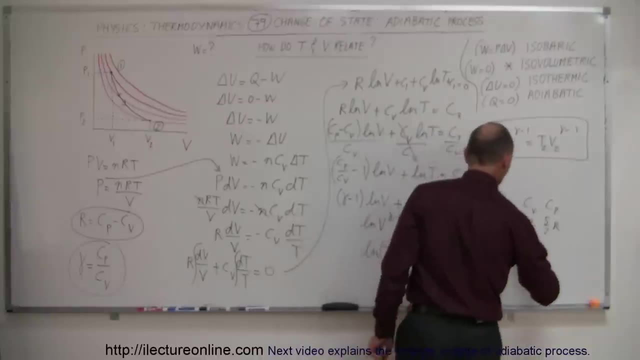 and C sub P is 5 over 2 R for a diatomic gas, I mean for a monatomic gas. For a diatomic gas, diatomic C sub V is 5 over 2 R and C sub P is 7 over 2 R. 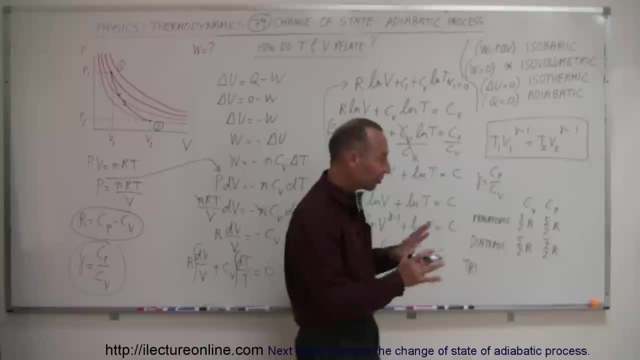 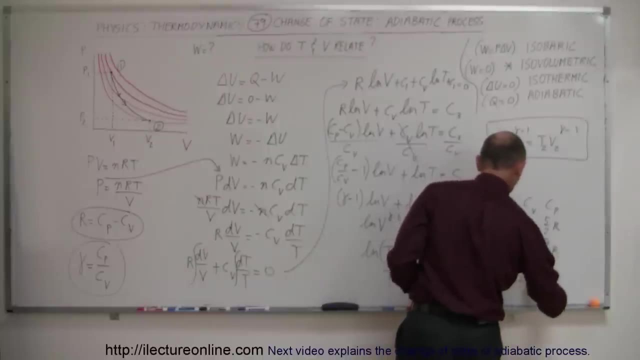 And for a triatomic gas, and of course these are approximate numbers. real gases differ slightly from real gases, but it's good enough for our purpose. Triatomic C sub V is 7 over 2 R and C sub P is 9 over 2 R. 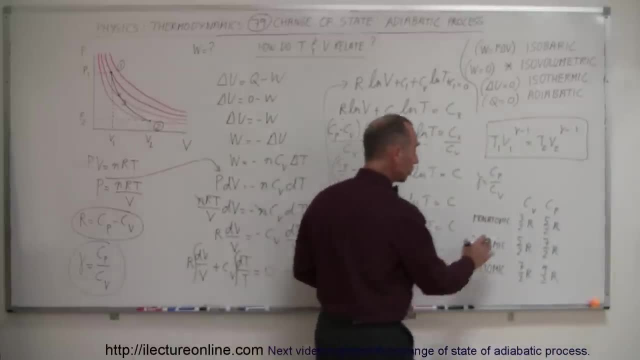 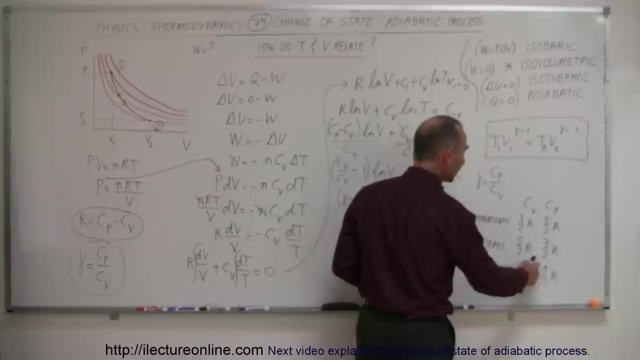 And again, those are approximate numbers. So when we take the ratio notice, for a monatomic gas the ratio would be 5 over 3, for a diatomic gas it would be 7 over 5, and for a triatomic gas it would be 9 over 7.. 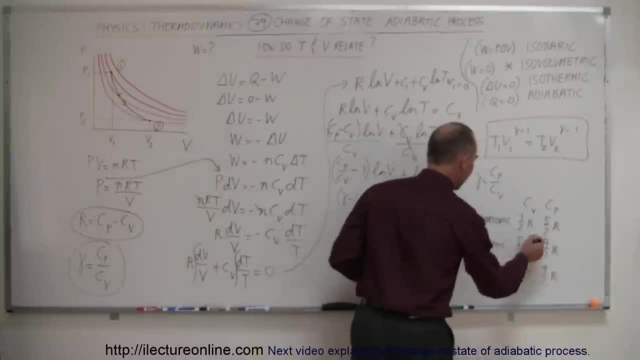 So just so you can see how that works, let's take the example of the diatomic gas for a moment. So we have 5 over 7 over 2 R. divided by 5 over 2, R is equal to: if we cancel that out, 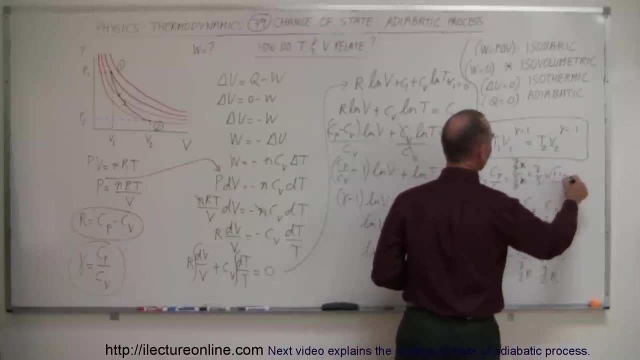 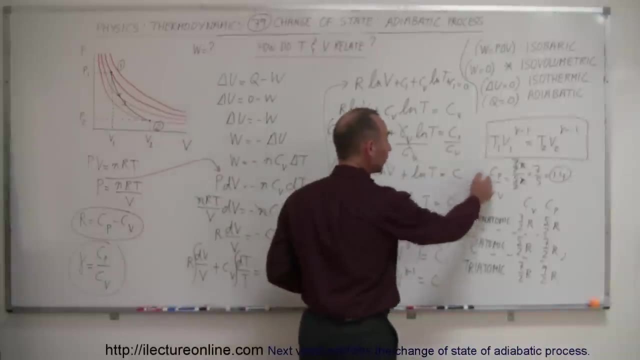 is 7 over 5, or 1.4.. So there you can see that once you know what gas you're dealing with, you can figure out the gamma, because you can figure out the ratio, and then you can plug that in here. 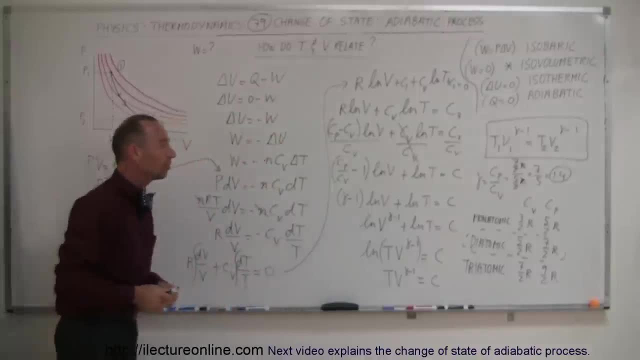 and get the relationship between temperature and volume for any adiabatic process and that will help you eventually find the work done in the gas and let me find out where that is. that would be this thing right here, so that allows you to find the difference in the temperature.